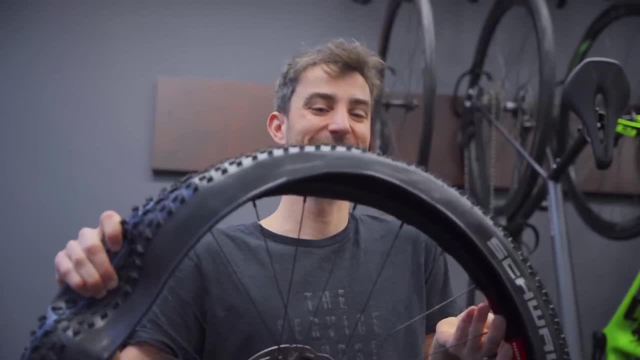 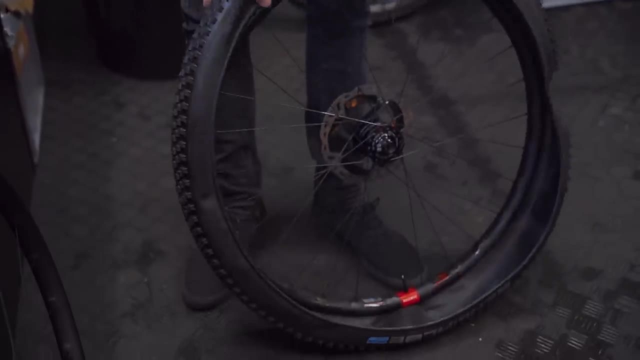 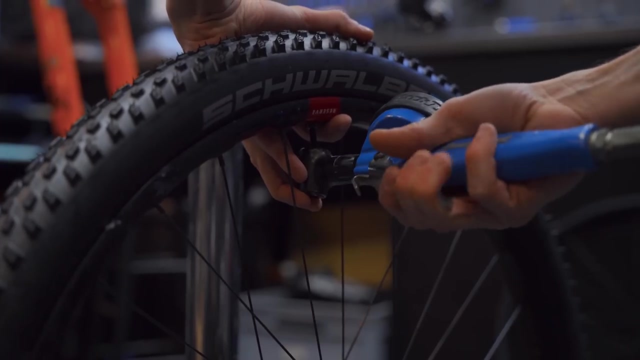 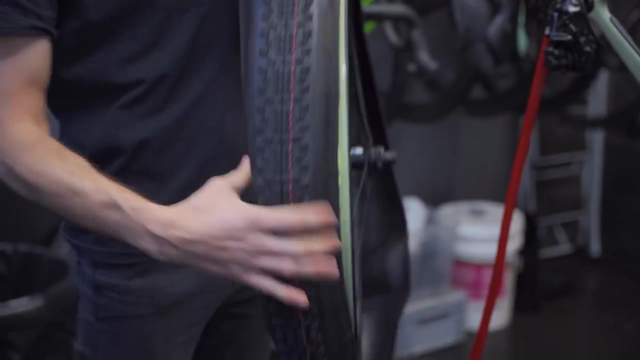 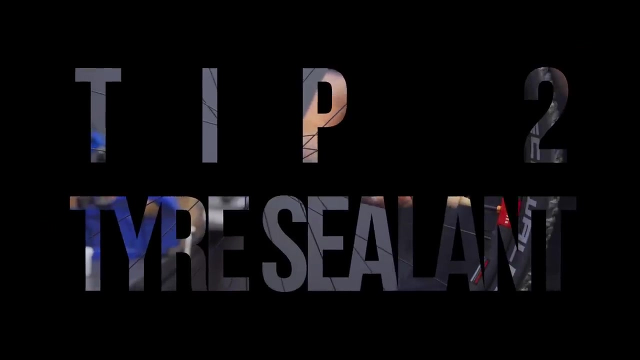 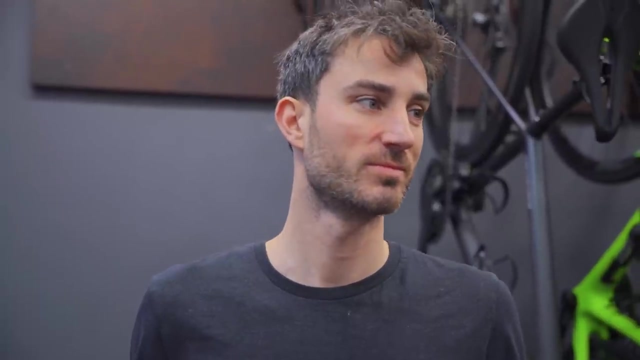 I put the sealant in before I pop the tyre. Oh, it's in my mouth: Schwalbe, Schwalbe, Schwalbe. If you can install the tyre without the sealant- first- essential- and then add the sealant. 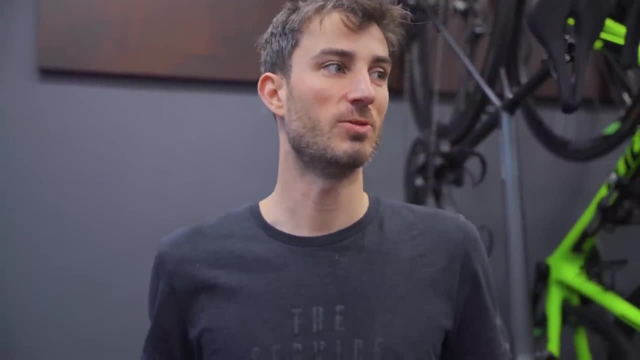 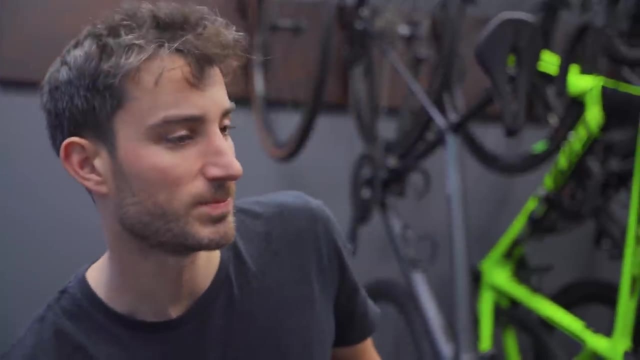 through the valve, Because sometimes things go wrong and you have the sealant and the tyre doesn't beep and it's a real mess. Although if you can't do it, you're going to have to do it like I showed you before. 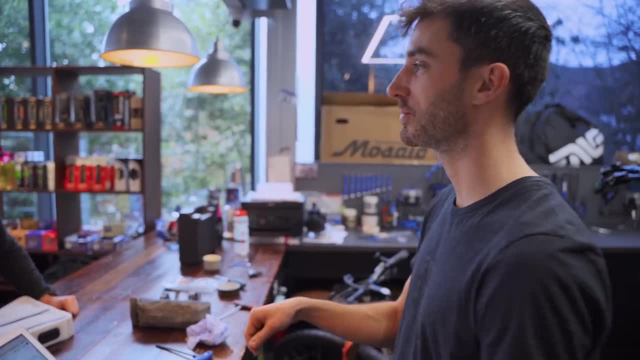 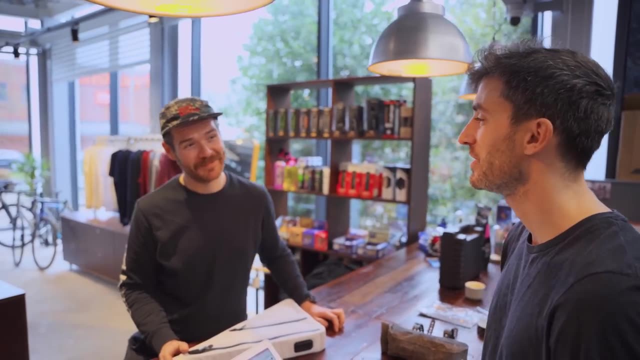 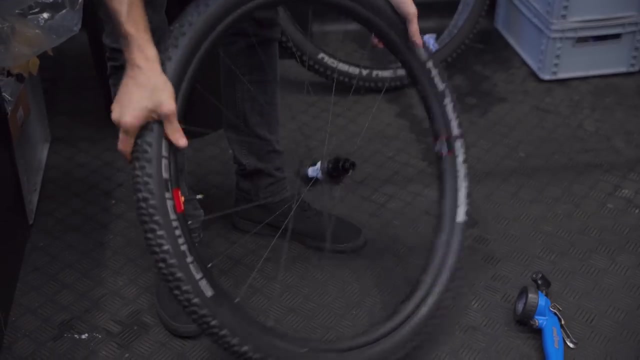 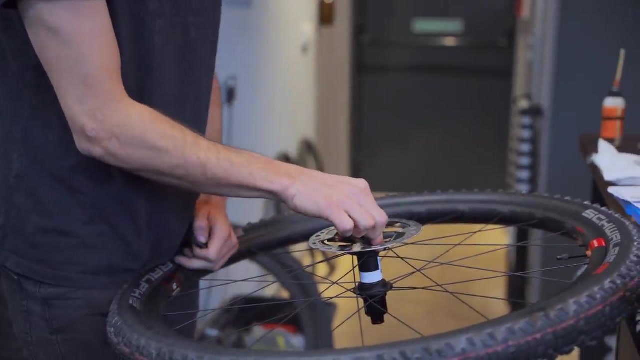 So put the sealant first, Because that valve doesn't allow to insert the sealant in the air. So this tip that I just gave doesn't always work. Now it's very essential. Do you want this aligned, Or do you want this not aligned? 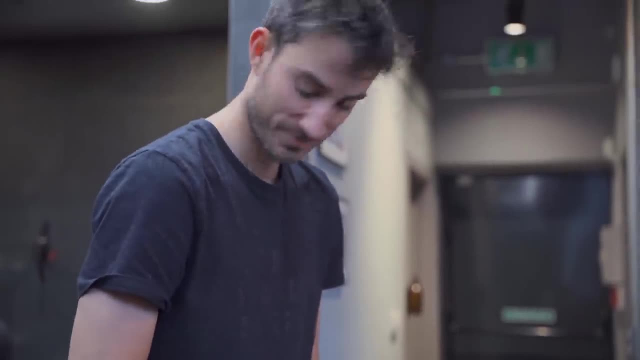 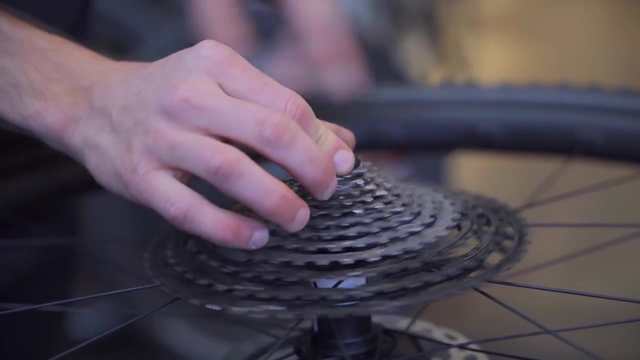 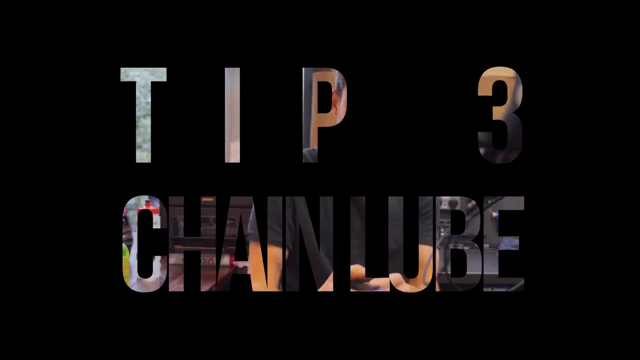 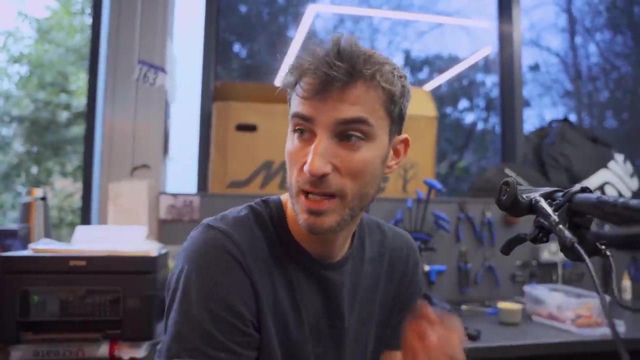 It's very important to me. This is very important to you. yeah, It is very important. Well, you can either apply lube straight away, Just make sure you don't really apply only on the rivets. Sometimes The main thing for water displacement is to use some sort of Teflon spray, like you. 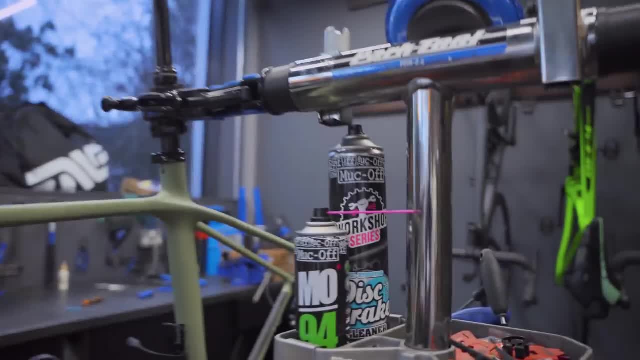 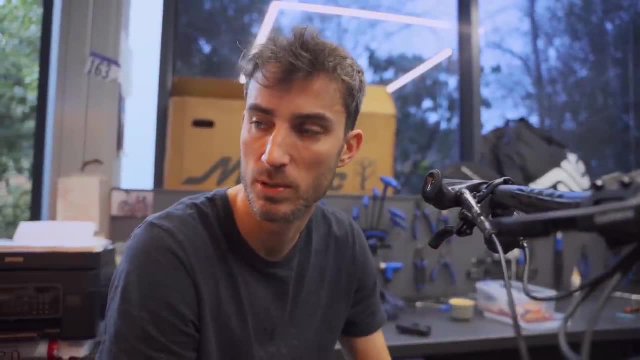 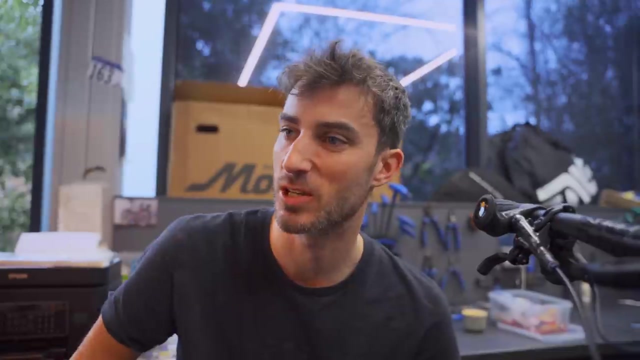 know the Markov thing on the chain. That's not a trust. Then you let it dry out and then you apply the lube that you want. Do you wax it or do you lube it? I'm a luber, You're a luber. 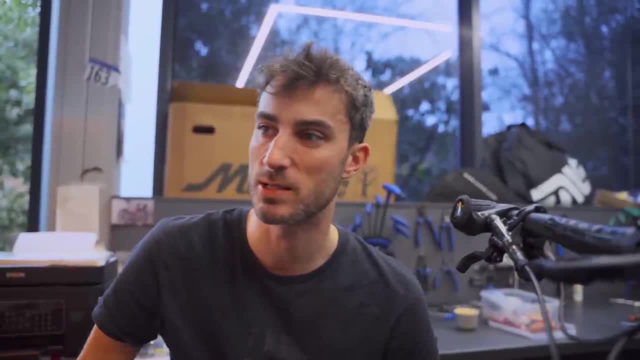 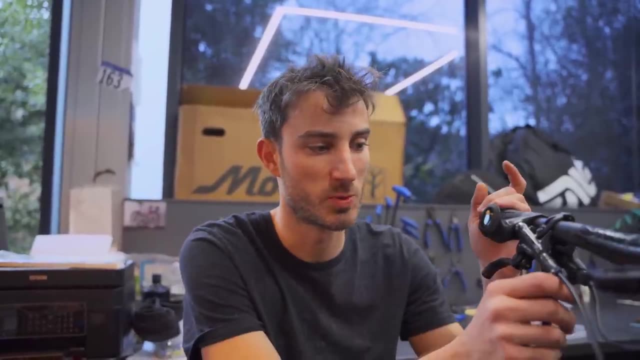 There's a lot of gunk that sticks to the chain when you use wax. Not that a normal lube doesn't, It's just. But it also depends on the weather. you know, A wet lube always works and a dry lube only works every now and then. 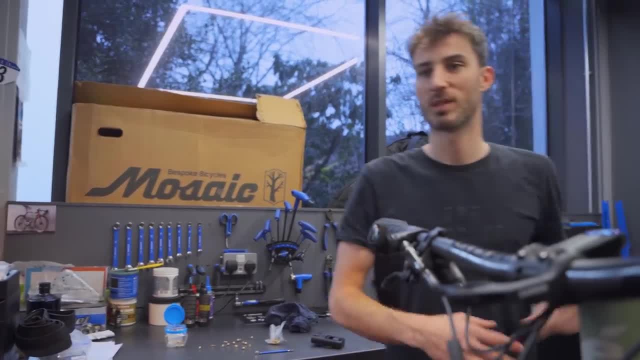 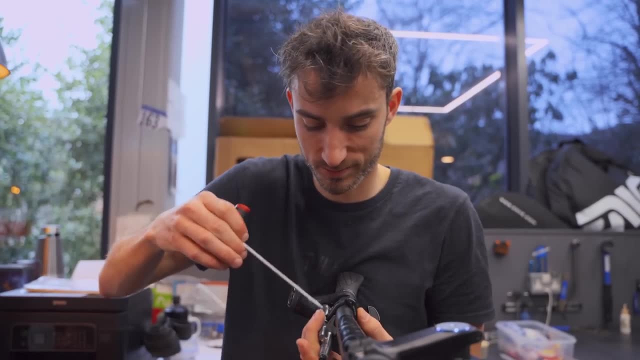 Every now and then, especially, you know, for the winter, wet lube. it's basically six months of the year wet lube In the UK, In the UK at least, And then, well lube every now and then. 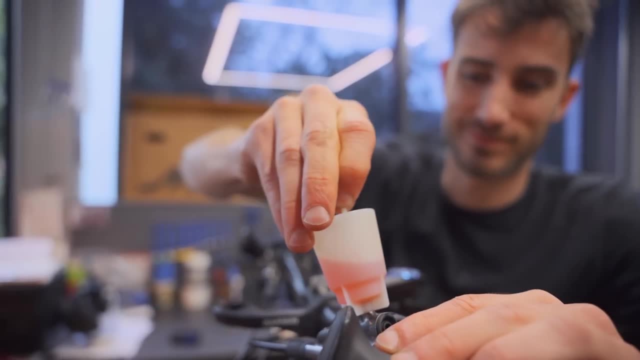 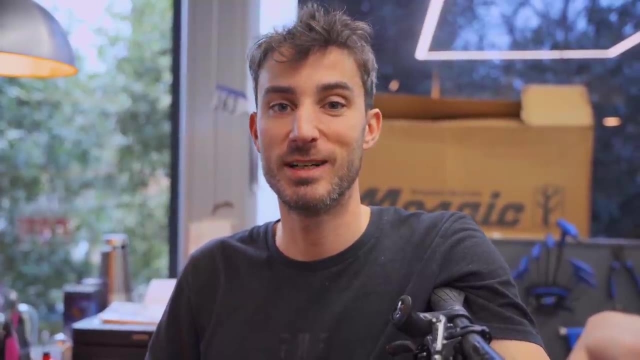 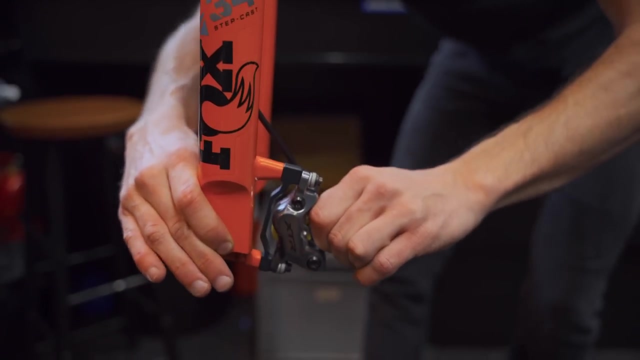 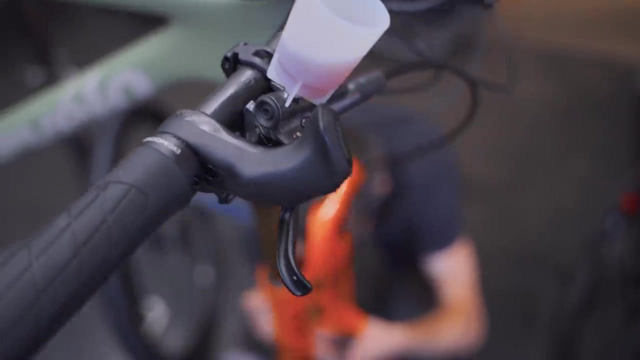 Very, very, very old, but very, very old lube Bleeding brakes. It requires specific tools, handling oil and a little bit of knowledge. so take it to your local bike shop. That's a tip. Your car has to get down like this: 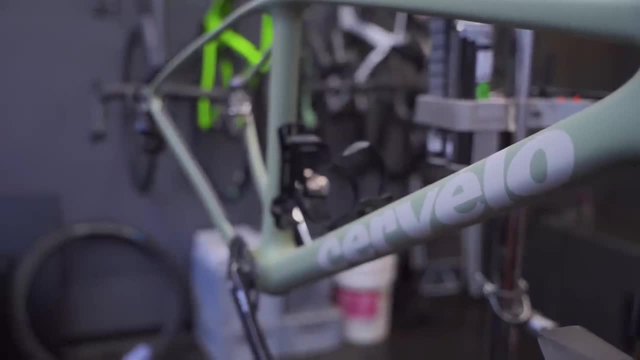 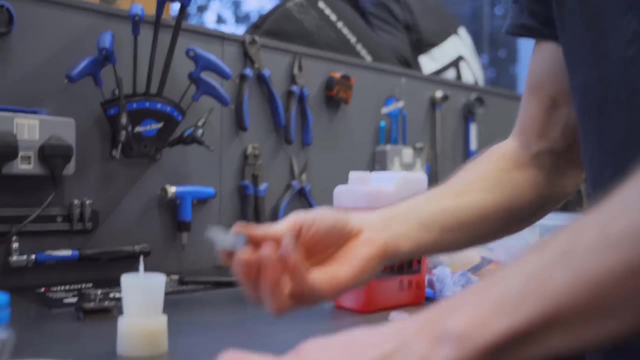 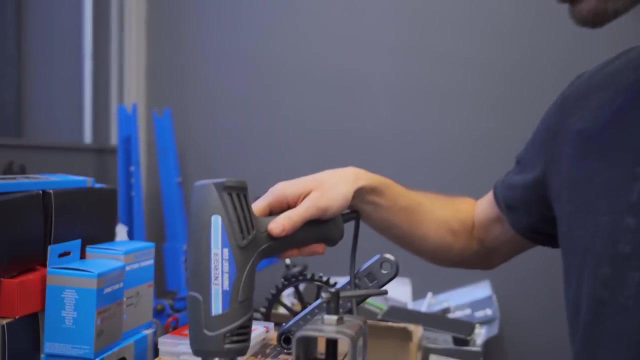 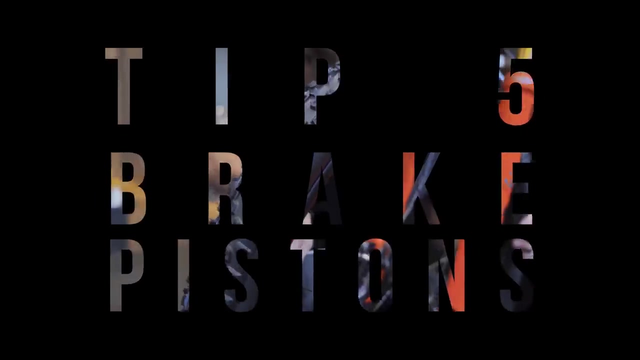 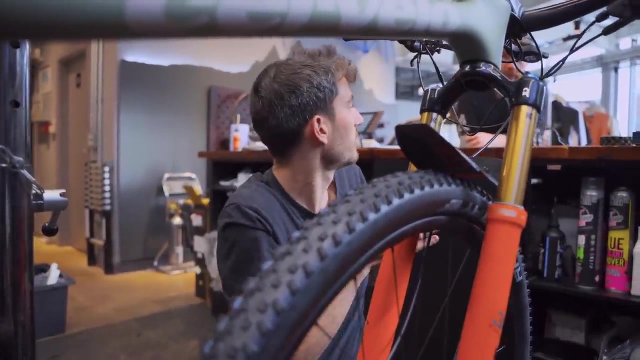 You do not know. Oh gosh, That's the problem. I've got something better than a lighter. I've got a heat gun. This is my best friend. Yeah, make sure that the pads, the pistons, are fully retracted. Sometimes they are a little. 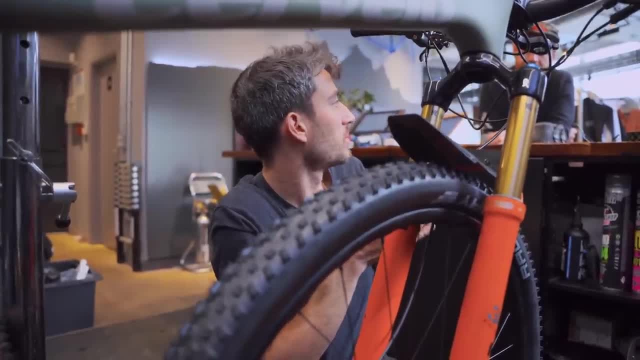 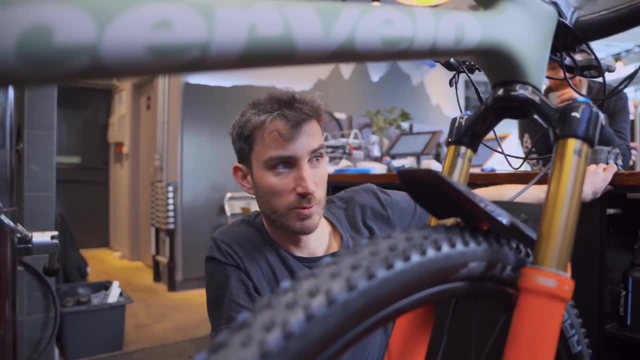 bit out and there is a little bit more space that you can get by pushing the pistons fully back inside. They should always be done, though, like gently and with a plastic tyre lever. That's the best thing. Don't do it with metal, don't do it with tools, basically. 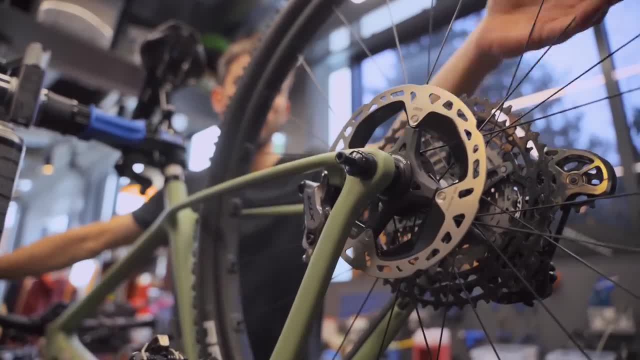 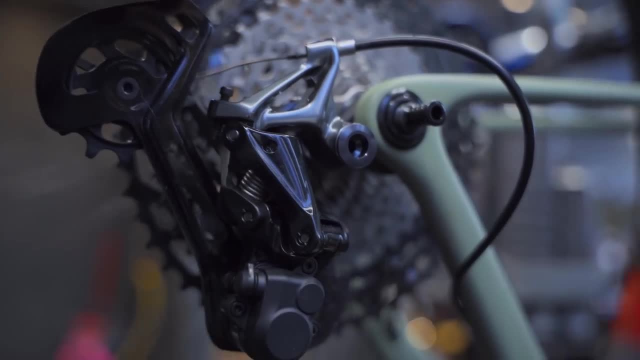 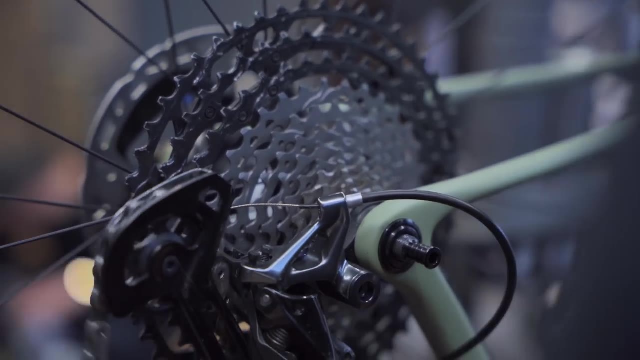 just use some plastic tyre levers. It's a nice sounding hub, Nice and quiet. One thing about the quicklimb: if you don't have pliers, just take it above the chainstay and then hold the wheel and it clicks on. 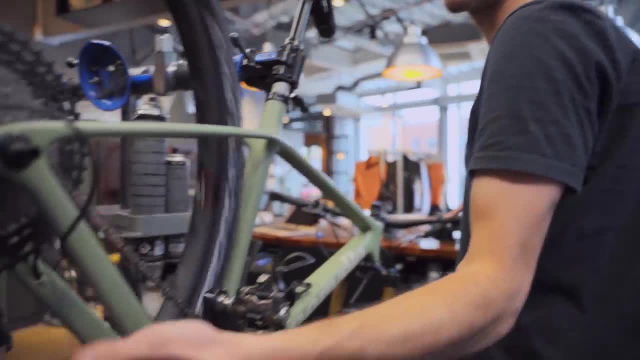 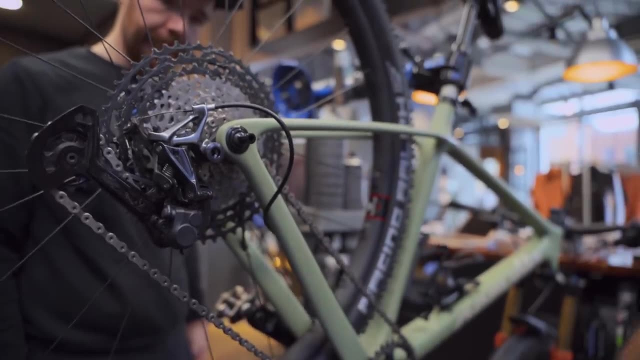 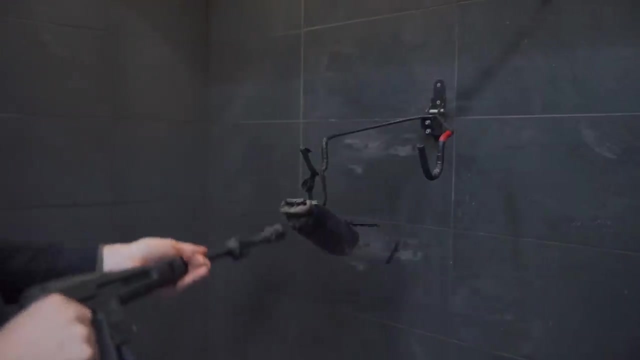 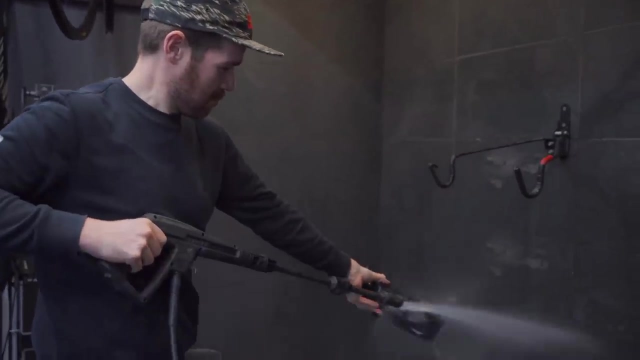 That is a good tip. If it's here, obviously there is no tension here. but if you take it to above the chainstay, just hold the wheel and click it in, You've got a job. It's really satisfying. It's really satisfying, yeah. 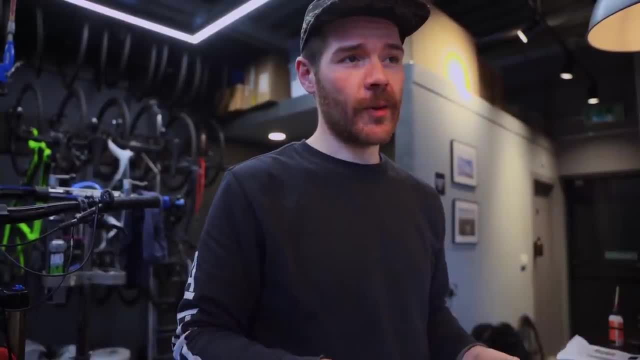 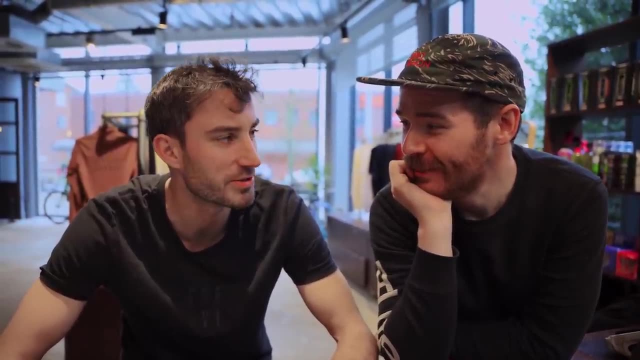 You didn't have to give me a t-shirt. I'd wear a medium if I was going to wear one, though, We say the same, Cervelo. I know I say the R, you don't say the R. Why don't you say the R?